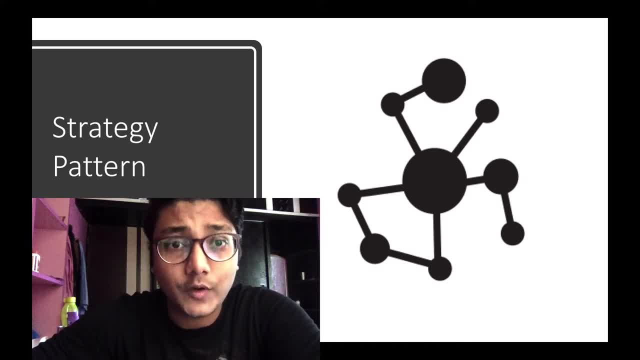 Good morning everyone. my name is Chiranjeevi and in today's video we are going to discuss the strategy design pattern. So the strategy design pattern is a straightforward design pattern and it's the simplest design pattern in the behavioral category. So let's have a look at the definition. 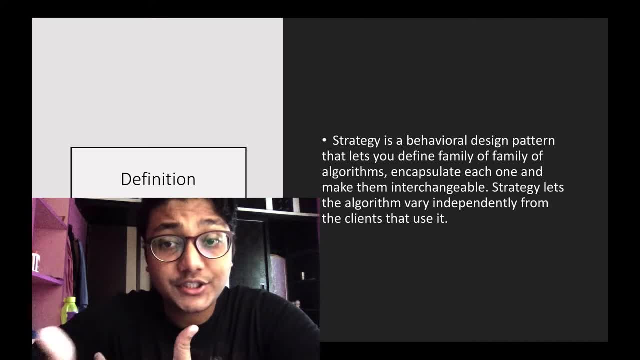 for the strategy design pattern. So strategy design pattern is a behavioral design pattern that lets you define family of algorithms, encapsulate each one and make them interchangeable. Strategy lets the algorithm vary independently from the clients that use it. So here's the idea: whenever you are using a particular algorithm to do a job, there can be multiple flavors of that. 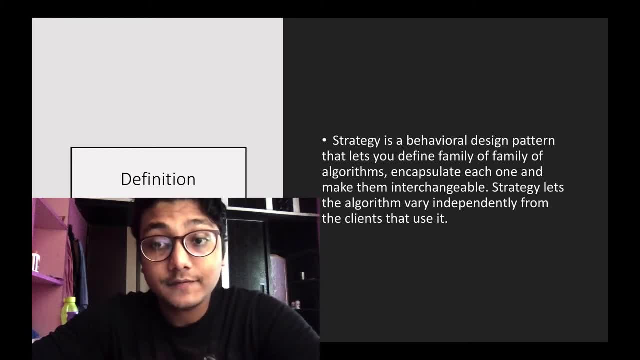 algorithm which can give you the same result. So, instead of coupling your code tightly to the algorithm being used, you can use the algorithm to do the same thing. So, instead of coupling your code tightly to the algorithm being used, what strategy design pattern suggests you to move that algorithm to a different class? 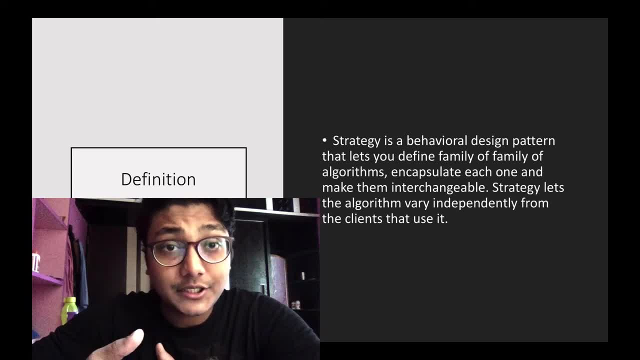 and encapsulate it using an interface and make it interchangeable with all the other flavors of the algorithm which you already have. Let's say we have sorting. The problem is sorting and we have different kinds of sorting strategies, like we have bubble sort, we have merge sort. 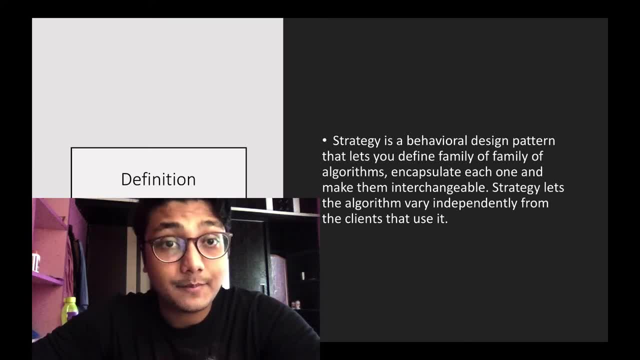 we have quick sort. All these sorting strategy gives us the same result, But the way we implement bubble sort and the way we implement merge sort is different, but the end result is the same. So these algorithms fall under the family of sorting algorithms and they 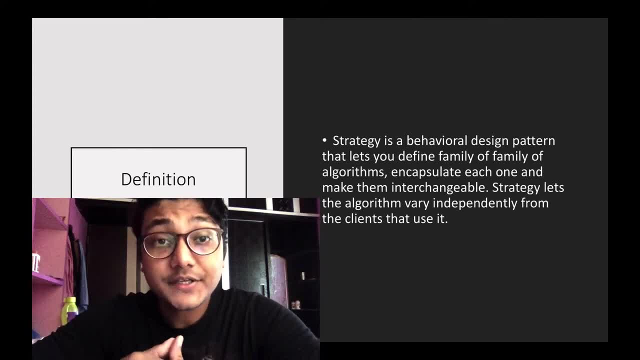 can be interchanged with each other. So instead of tightly coupling our code with our bubble sort algorithm, what we can do is create a sorting interface and inject different kinds of sorting algorithms and make them interchangeable with each other. So that's what strategy design pattern is. It's the simplest design pattern. 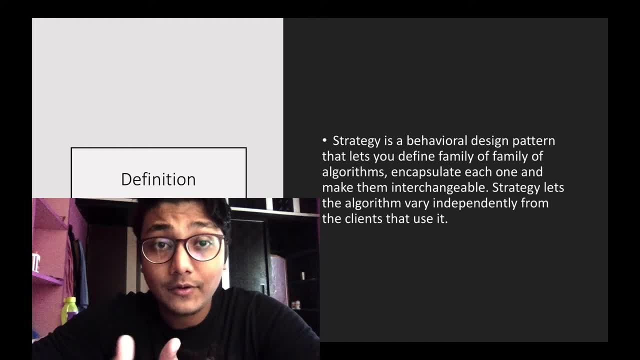 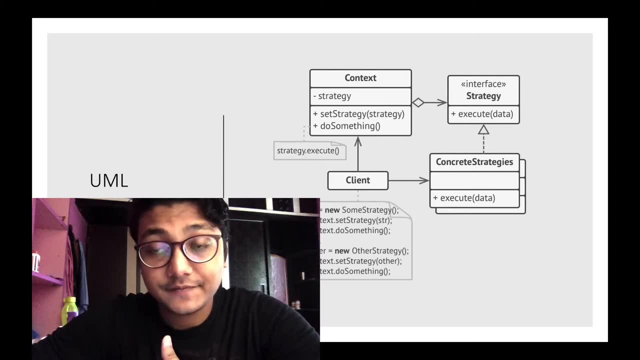 in the behavioral category. Let's have a look at the UML diagram. The UML diagram is also a quite straightforward thing. So we have a strategy interface which has this execute method and the concrete strategies actually implement this strategy interface and give the implementation for. 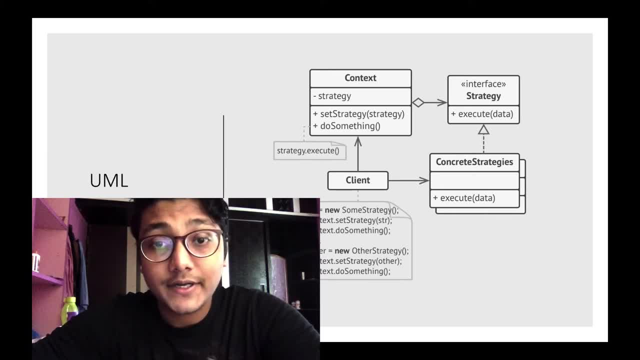 their own algorithms. We have a context which has a strategy and we have a method to set this strategy and execute that. So whenever we want to change the strategy, what we can do is we can use the set strategy method to change the strategy And at the end, the client will have this reference to this context. object: 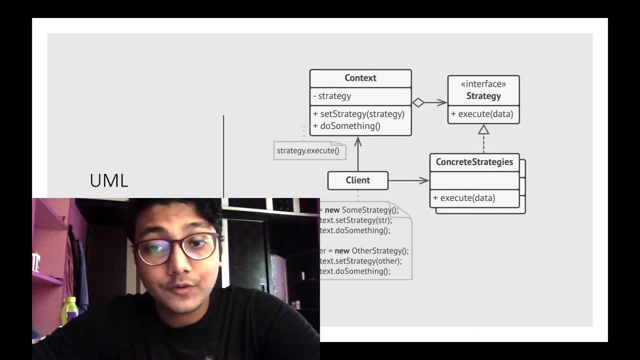 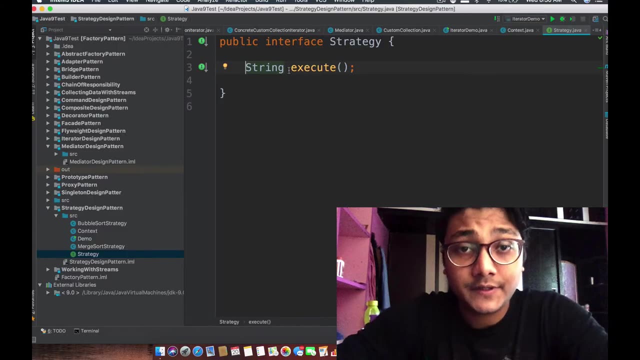 and it will inject one of its sorting strategy, whatever we want to inject, and it will call the do something method on the context object to execute this strategy. So that's what the UML diagram is. Let's quickly go ahead and take a look at the coding example. So our coding example is: 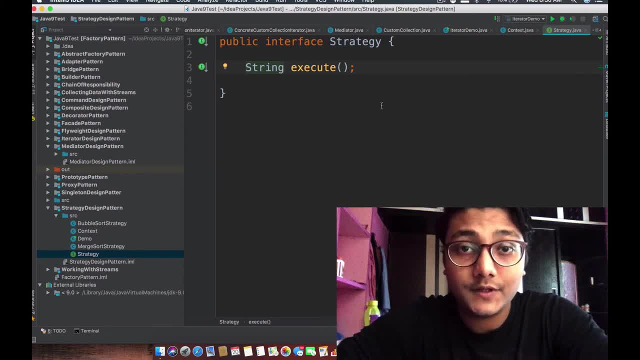 also similar to the UML diagram. It's kind of a one-to-one mapping. with the UML diagram We have an interface called strategy, which has this execute method and all those concrete strategies, be it your sorting algorithms or string manipulation algorithms or any algorithms or graph algorithms. 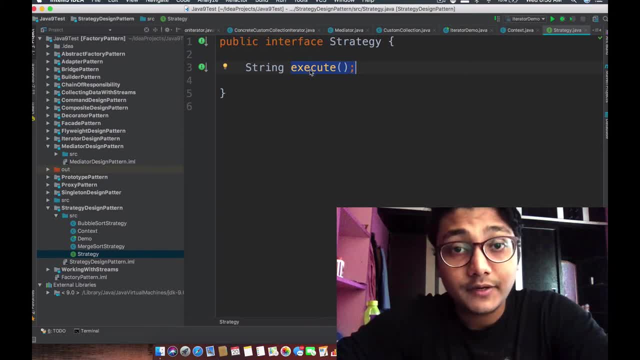 let it be graph traversal algorithms. So, whatever the result you require, the family of algorithms should provide the same result and all these separate member in the family can be encapsulated in the same way. So in this example, I am using this strategy interface by implementing their. 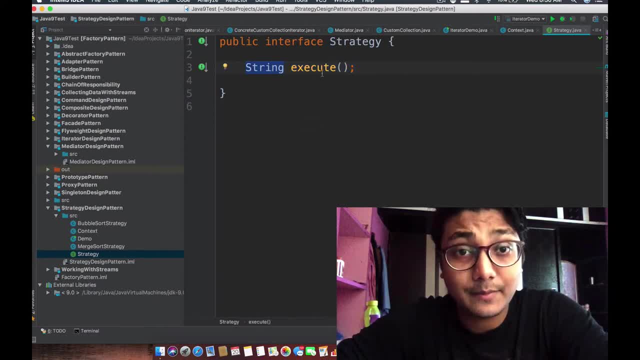 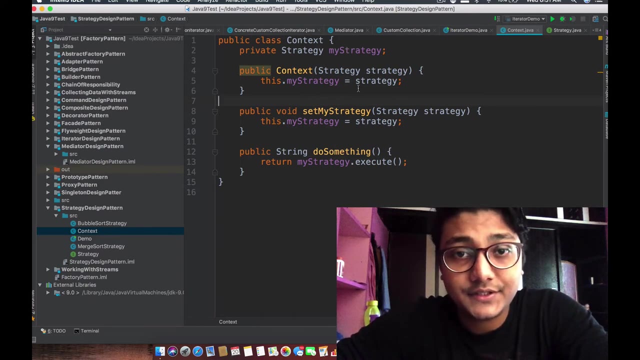 own version of that same algorithm and returning the result. So here to make to simplify this example, I have I am returning string as a result and not taking any parameters at all, And here we have our context object. In the context object we have a reference to our strategy. We are 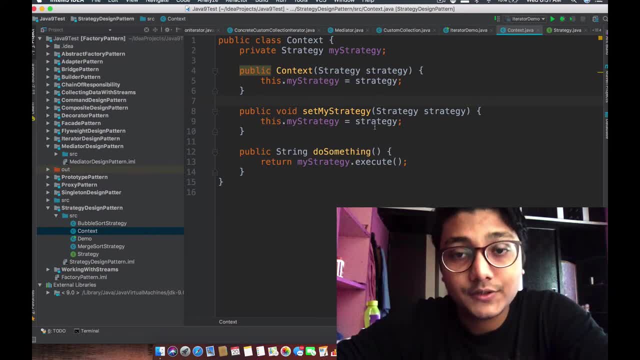 setting the strategy in the constructor and we have a set my strategy method to actually change the strategy for that algorithm. We can change it with this method, with the help of this method, And whenever we want to execute this strategy, we will call this do something method. Let's go to. 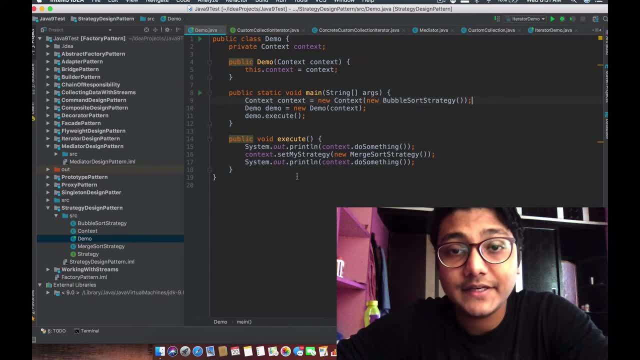 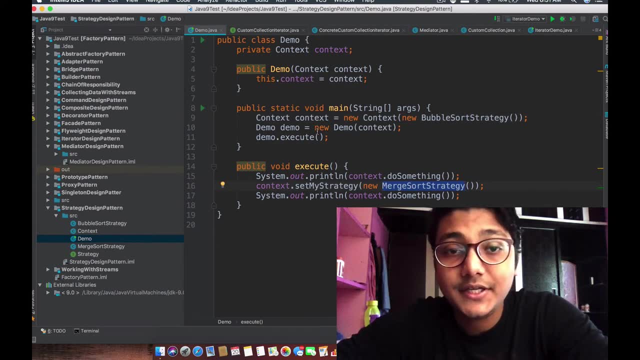 our demo method. So I have created two strategies: One is called the bubble sort strategy and one is called the merge sort strategy. So I'm instantiating this context object with bubble sort strategy and calling execute method on it. Calling the execute method on it actually invokes this method, which is calling the do something.